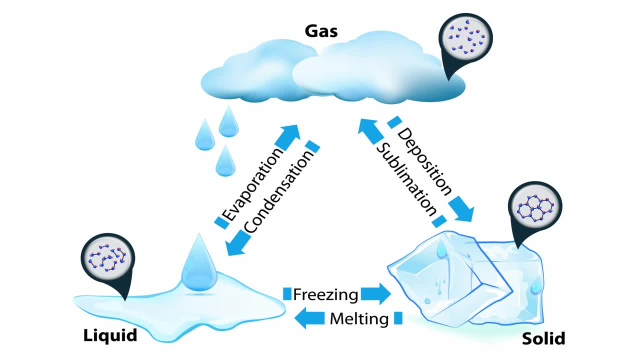 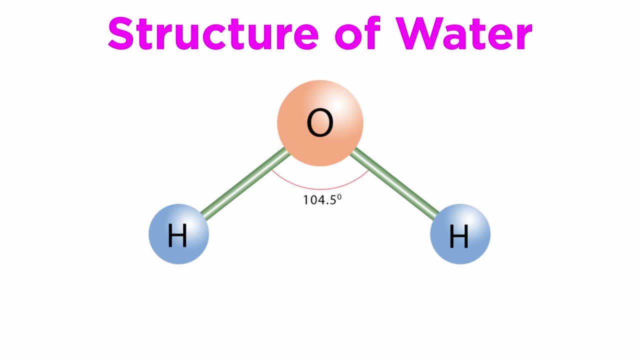 be readily found in three physical states: solid, liquid and gas. As we remember from our study of chemistry, water or H2O is made up of two hydrogen atoms and an oxygen atom. What makes this seemingly simple compound so special is its polarity. There's a partial positive charge on one. 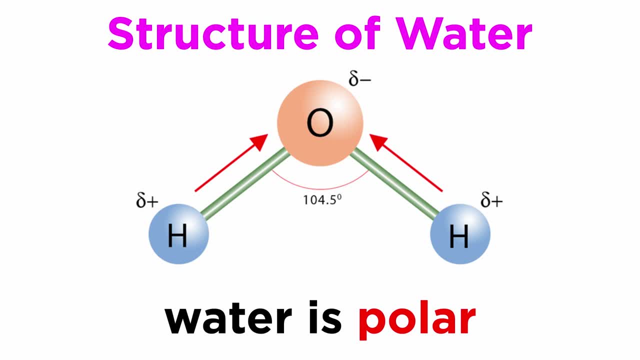 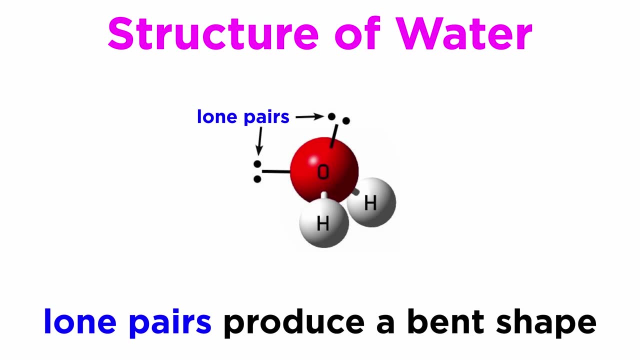 side and a partial negative charge on the other due to the polar OH bonds. The presence of two lone pairs of electrons on the oxygen atom gives water its bent shape, resulting in the overall net dipole. One water molecule attracts another via hydrogen bonds, and this is what 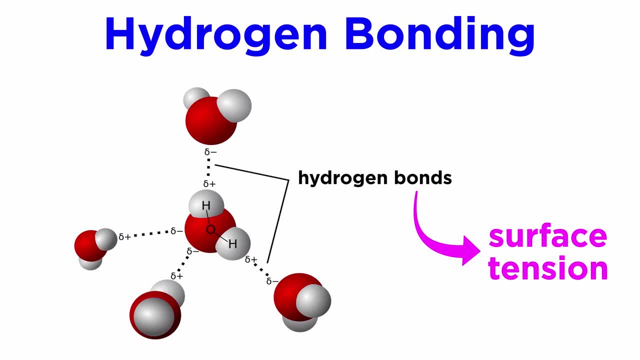 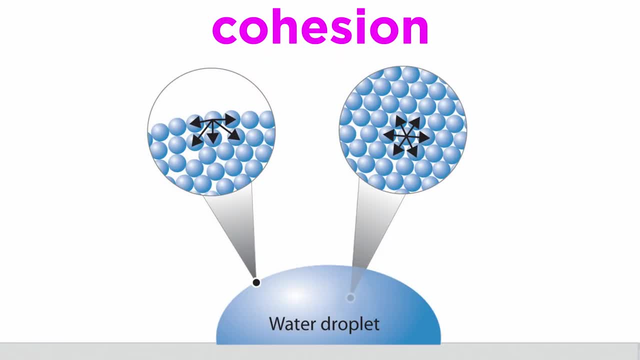 creates the hydrogen atom. The hydrogen atom is made up of two hydrogen atoms and the oxygen atom creates surface tension in a group of water molecules. Next time it rains, check out all the droplets that form when the water comes into contact with a waterproof jacket, Specifically, 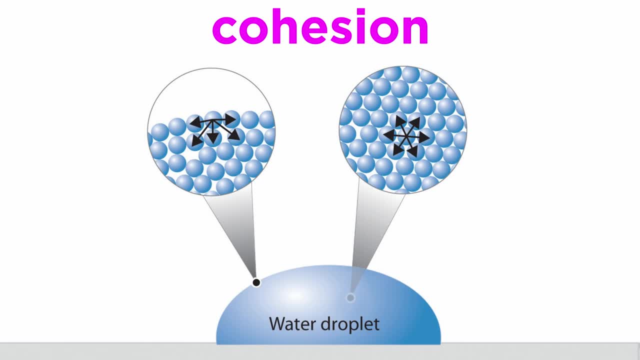 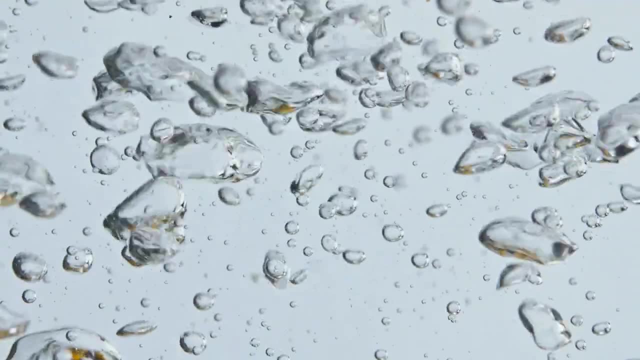 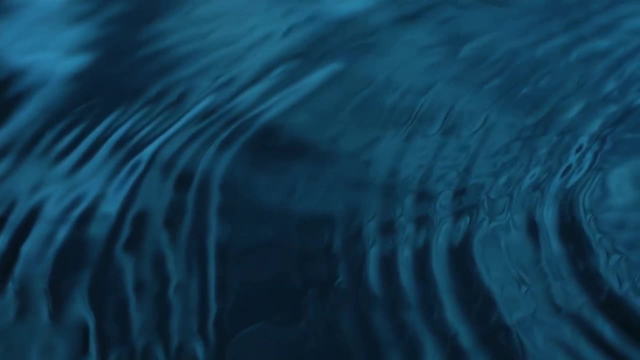 the bonding that makes the water molecules stick together is called cohesion. This property helps plants take up water at their roots. Cohesion also contributes to water's high boiling point, which helps animals regulate body temperature. More on the physical properties of water in the general chemistry series. 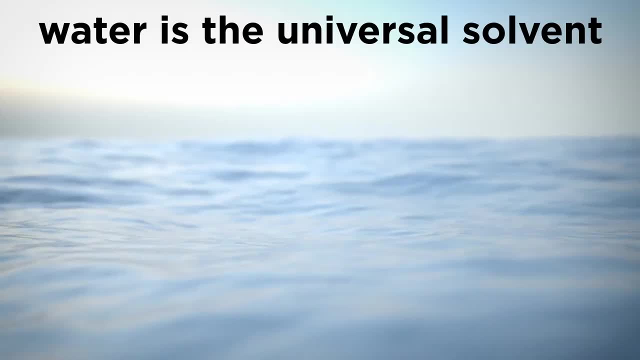 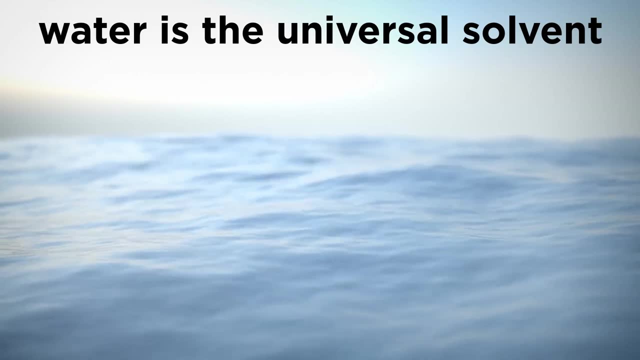 Given that water can dissolve a wide variety of molecules, it is known as the universal solvent. It's this ability that makes water such an invaluable life-sustaining force. On a biological level, water's role as a solvent helps cells transport and use. 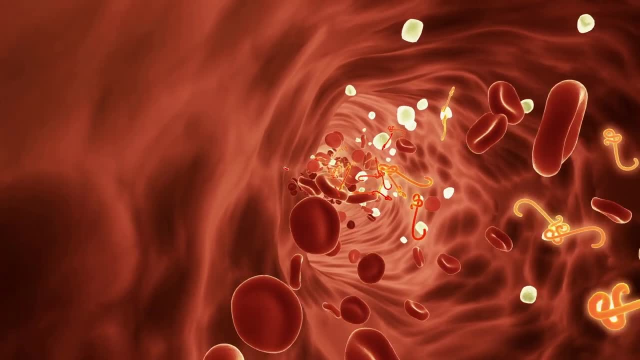 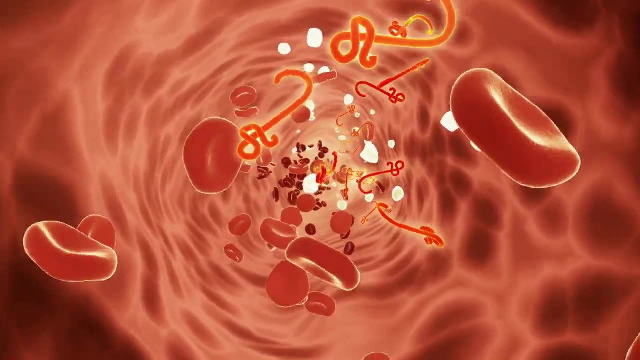 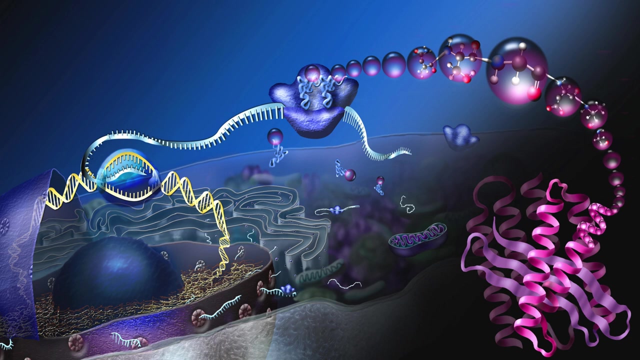 substances like oxygen or nutrients. Water-based solutions like blood help carry molecules to necessary locations, like oxygen for respiration. Water also allows everything inside cells to have a right shape at the molecular level, As shape is critical for biochemical processes. this is also 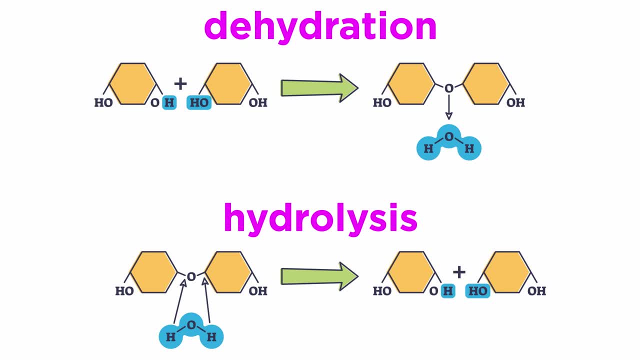 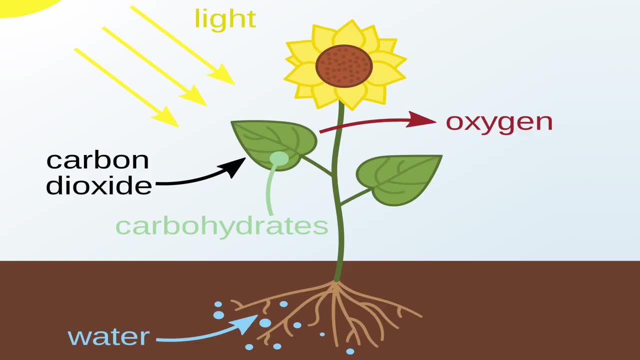 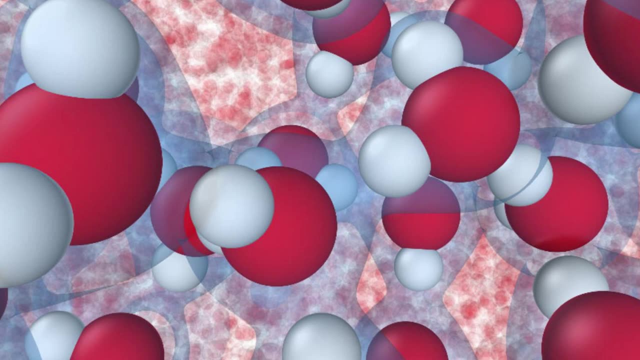 one of water's most important roles. Water is directly involved in many chemical reactions to build and break down important components of the cell. Photosynthesis, the process in plants that creates sugars for all lifeforms and the oxygen we breathe, requires water. It's pretty. 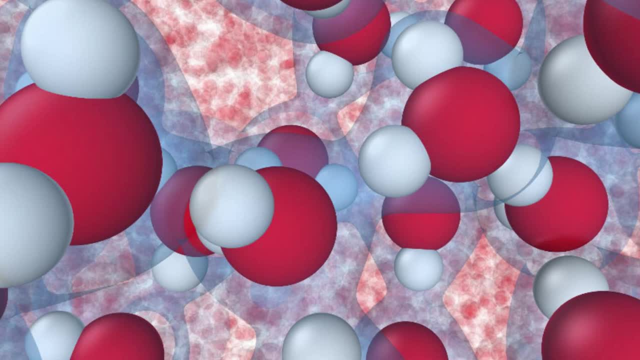 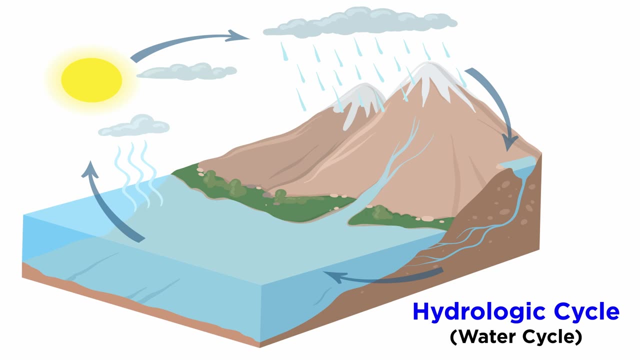 amazing how a simple molecule is so universally important for organisms with diverse needs. Water is distributed and recycled through the biosphere via the hydrologic cycle, which involves the circulation of water in the Earth-atmosphere system in a continuous manner. It has no beginning or end. But let's start in the ocean, as this is where 70% of Earth's water. 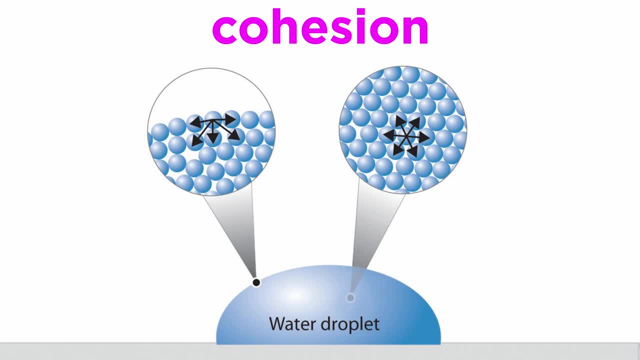 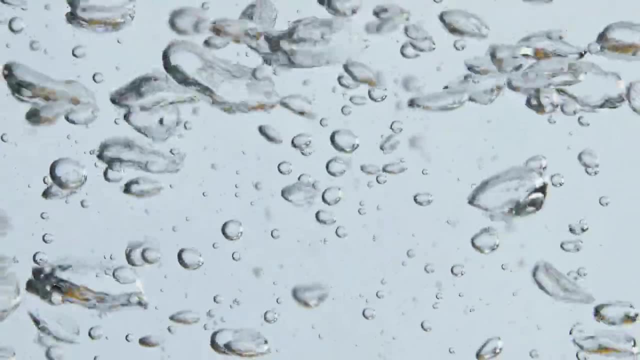 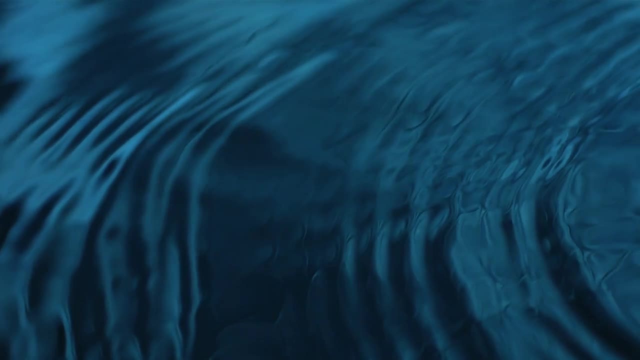 makes the water molecules stick together is called cohesion. This property helps plants take up water at their roots. Cohesion also contributes to water's high boiling point, which helps animals regulate body temperature. More on the physical properties of water in the general chemistry series. 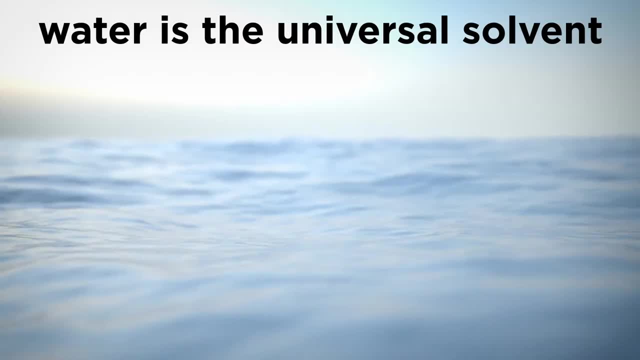 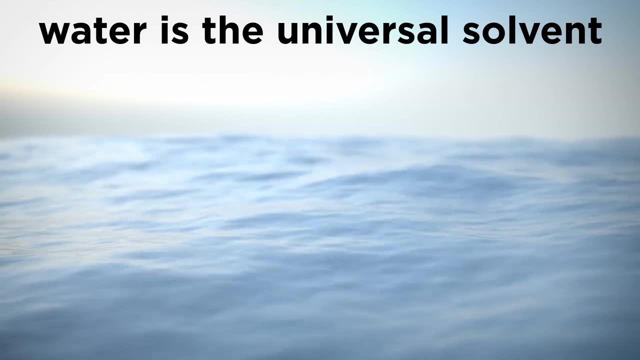 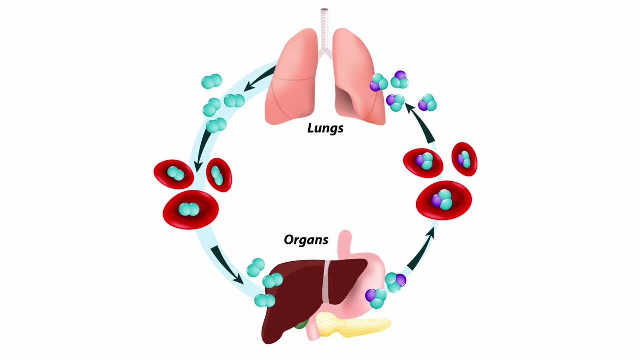 Given that water can dissolve a wide variety of molecules, it is known as the universal solvent. It's this ability that makes water such an invaluable life-sustaining force. On a biological level, water's role as a solvent helps cells transport and use substances like 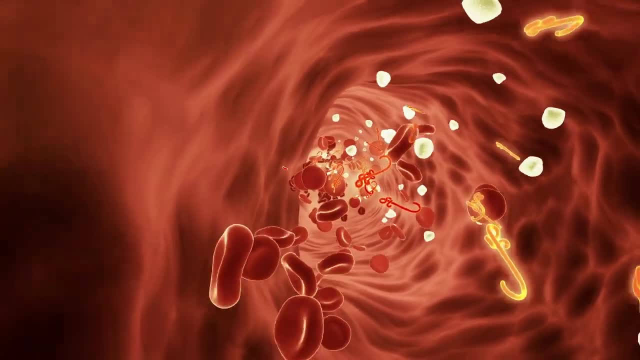 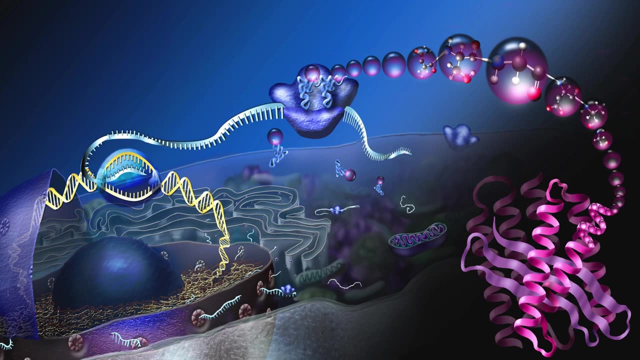 oxygen or nutrients. Water-based solutions like blood help carry molecules to necessary locations like oxygen for respiration. Water also allows everything inside cells to have a right shape at the molecular level, As shape is critical for biochemical processes. this is also one of water's most important roles. Water is directly involved in many chemical reactions to 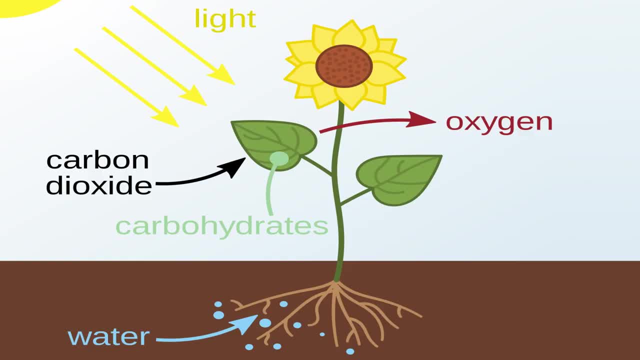 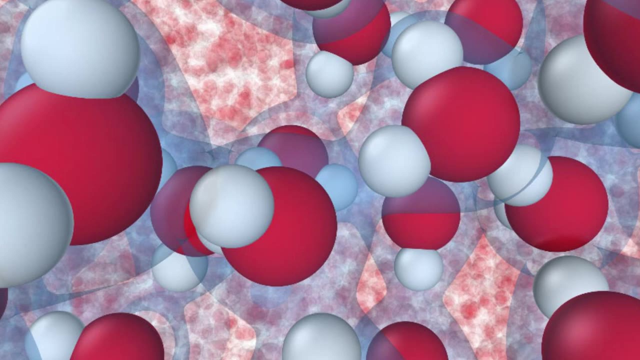 build and break down important components of the cell. Photosynthesis, the process in plants that creates sugars for all lifeforms and the oxygen we breathe requires water. It's pretty amazing how a simple molecule is so universally important for organisms with diverse needs. 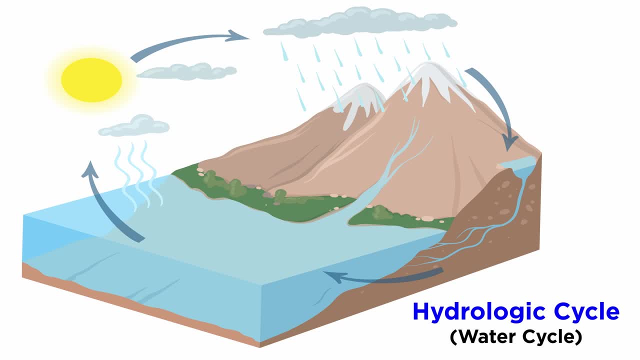 Water is distributed and recycled through the biosphere, via the hydrologic cycle, which involves the circulation of water in the earth-atmosphere system in a continuous manner. It has no beginning or end. But let's start in the ocean, as this is where 70% of earth's water 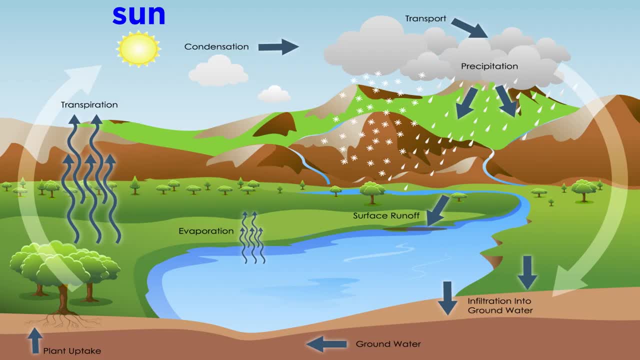 resides. The sun is the true driver of the hydrologic cycle, as it begins by heating the water in the oceans. Some of the water evaporates, turning from liquid to vapor. This water vapor is joined by water vapor from evapotranspiration. 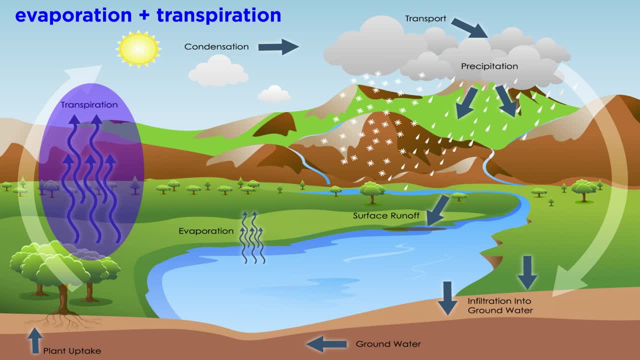 which is water that has either transpired from plants or evaporated from the soil. As this cumulative vapor rises into the air, it cools and eventually condenses into clouds. Air currents move clouds around the globe and eventually cloud particles collide, grow and fall out of the sky. 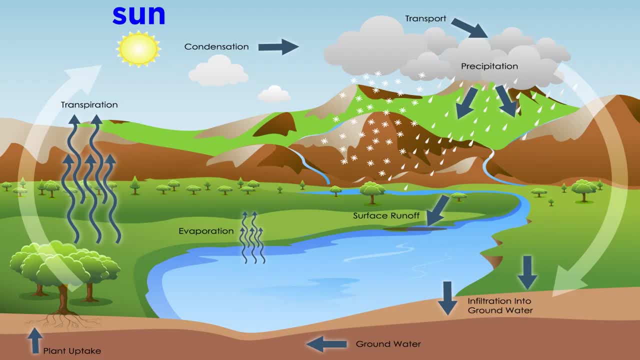 resides The sun is the true driver of the hydrologic cycle, as it begins by heating the water in the oceans. Some of the water evaporates, turning from liquid to vapor. This water vapor is joined by water vapor from evapotranspiration, which is water that is either. 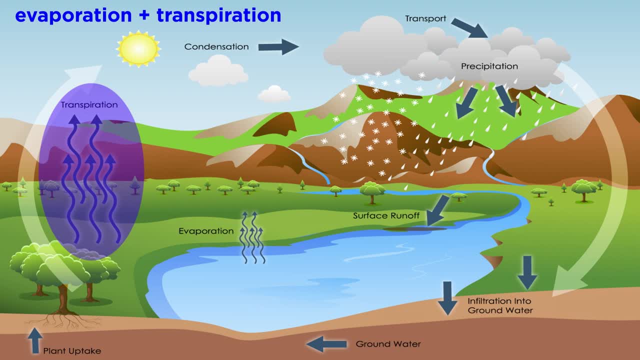 transpired from plants or evaporated from the soil. As this cumulative vapor rises into the air, it cools and eventually condenses into clouds. Air currents move clouds around the globe and eventually cloud particles collide, grow and fall out of the sky as rain, snow or hail known. 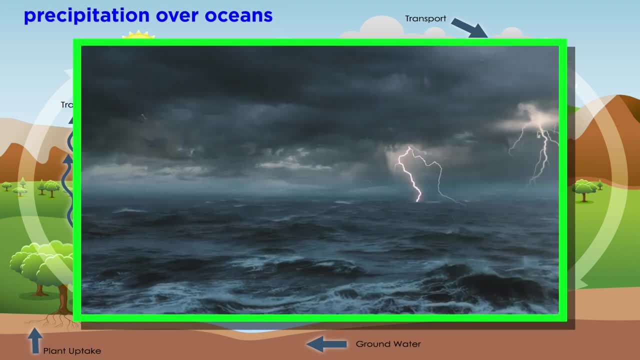 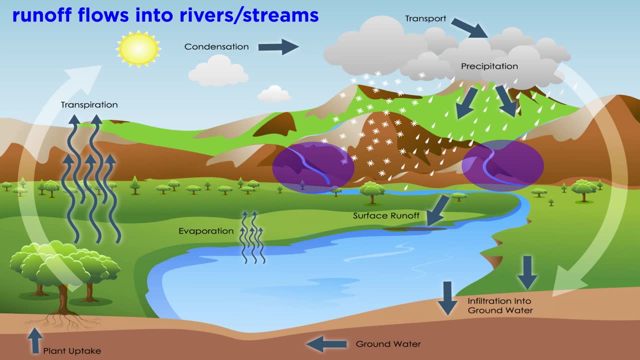 collectively as precipitation. Most of the water vapor is formed by evapotranspiration, which is the process of precipitation. Most precipitation falls back into the oceans. The precipitation that lands on the Earth's surface flows away from where it lands as runoff due to gravity. 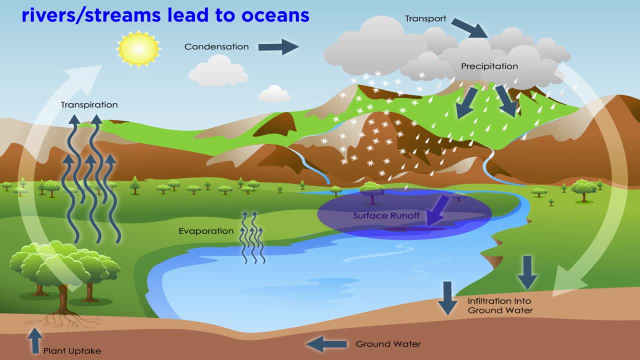 A portion enters rivers and streams, which eventually flow into the ocean, but the rest of the runoff and groundwater seepage can accumulate and get stored as freshwater in lakes. The runoff that doesn't flow into rivers soaks into the ground as infiltration and finds its way deep down underground into aquifers, water and water. The runoff that 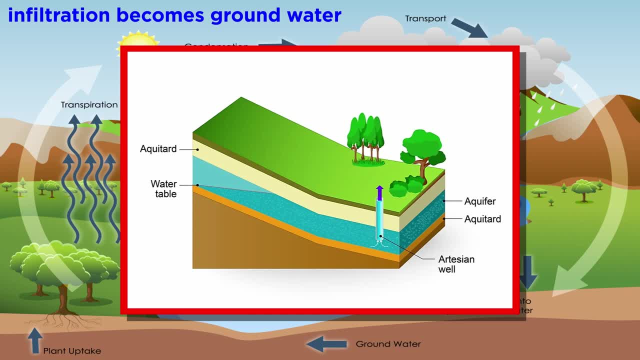 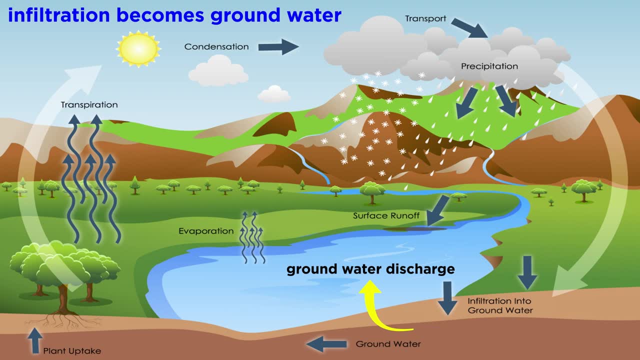 doesn't flow into rivers, soaks into the ground as infiltration and finds its way deep down underground into aquifers or saturated rock, which can store large amounts of freshwater for long periods of time. Infiltration that stays close to the surface can seep back into surface water bodies. 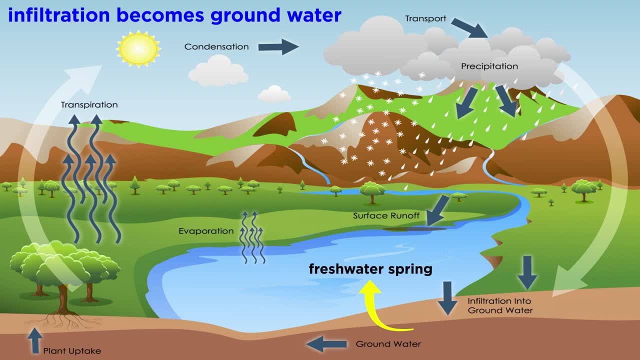 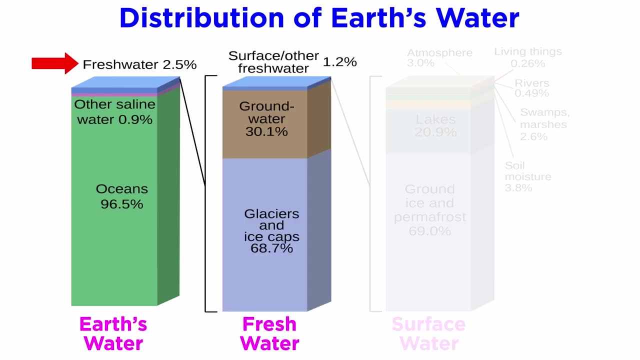 and the ocean as groundwater discharge, or it can emerge as freshwater springs. Of the world's total water, over 96% of it is salty. Of the total freshwater, over 68% is locked up in ice and glaciers, with another 30% of freshwater stored in the ground. 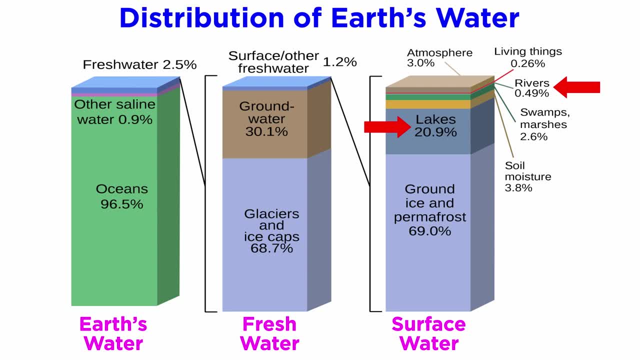 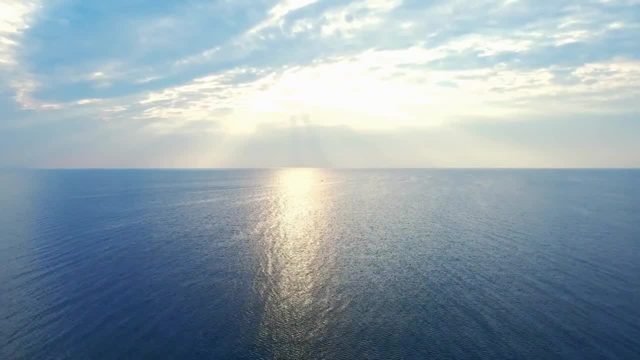 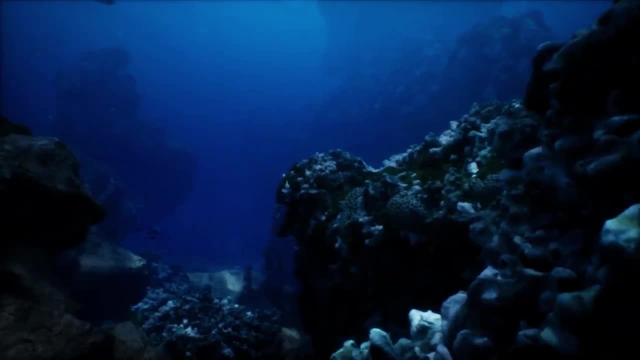 Rivers and lakes that we use and enjoy actually make up less than 0.01% of the total water on the planet. When it comes to the marine environment, these aquatic areas have high levels of dissolved salt and include the open ocean, deep sea, ocean and coastal marine ecosystems. 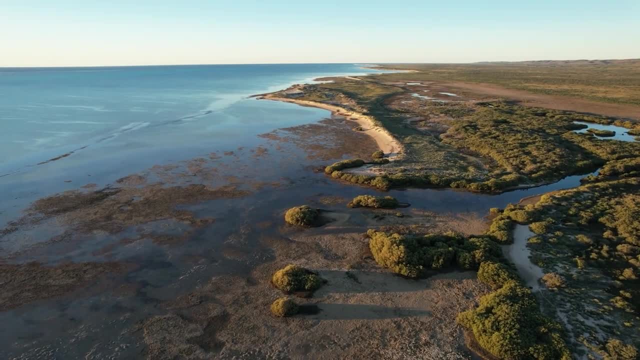 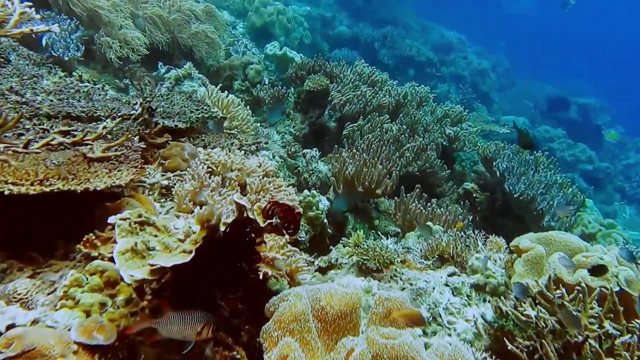 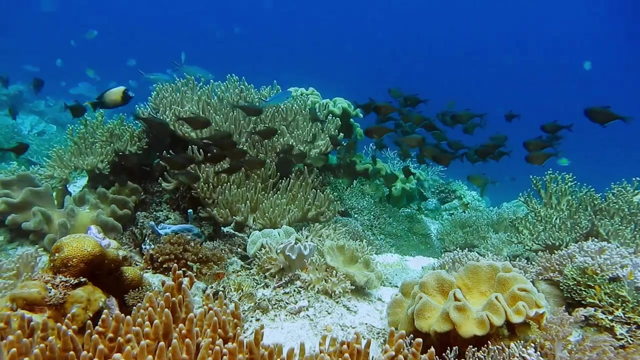 like coral reefs and estuaries where tides meet streams, Each has different physical and biological characteristics. Coral reefs, for example, are incredibly diverse marine ecosystems, which in total may account for a quarter of all ocean species alone. Corals are slow-growing, taking a long time to form. The fastest-growing coral grows 6 inches. 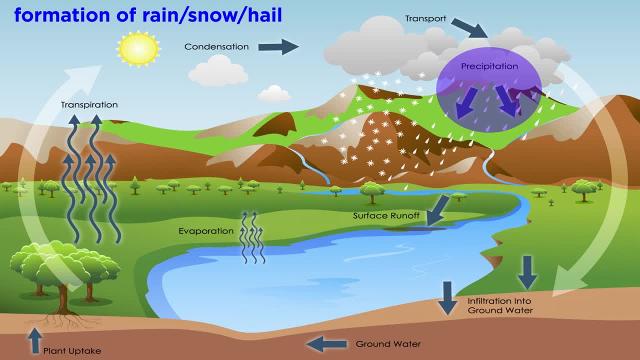 as rain, snow or hail, known collectively as precipitation. Most precipitation falls back into the oceans. The precipitation that lands on the Earth's surface flows away from where it lands as runoff due to gravity. A portion enters rivers and streams, which eventually flow into the ocean, but the rest of the runoff and groundwater seepage can. accumulate and get stored as freshwater in lakes. The runoff that doesn't flow into rivers soaks into the ground as infiltration and finds its way deep down underground into aquifers or saturated rock, which can store large amounts of freshwater for long periods of time. 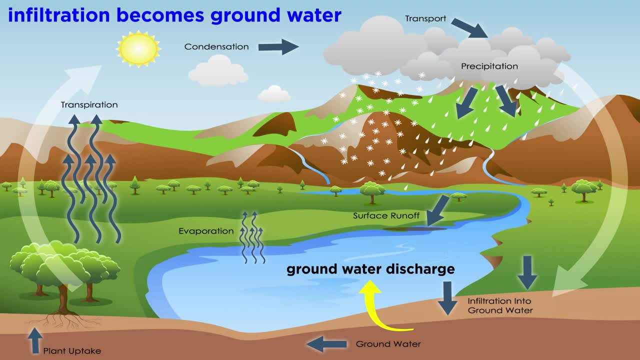 Infiltration that stays close to the surface can seep back into surface water bodies and the ocean as groundwater discharge, or it can emerge as freshwater springs. Of the world's total water, over ninety-six percent of it is salty. Of the total freshwater, 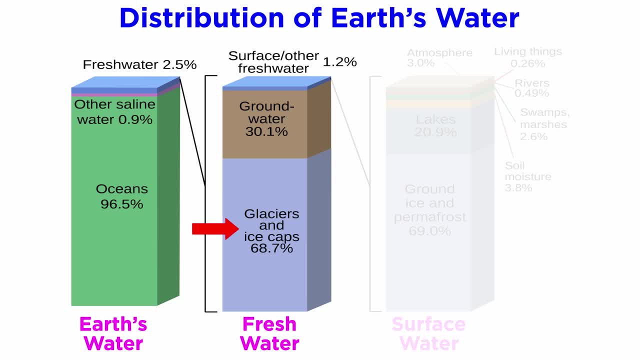 over sixty-eight percent of it is saltwater Of the total freshwater. over sixty-eight percent of it is salty Of the total freshwater- over sixty-eight percent of it is salty Of the total- is locked up in ice and glaciers, with another 30% of fresh water stored in the ground Rivers. 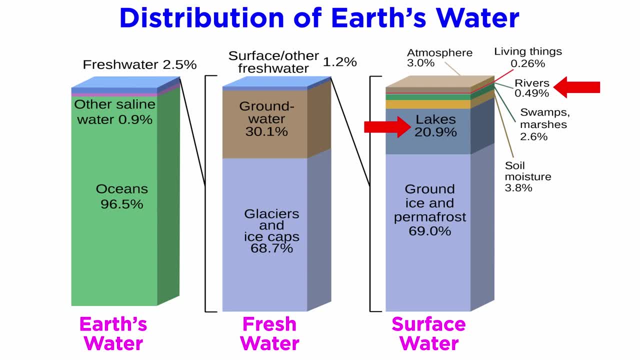 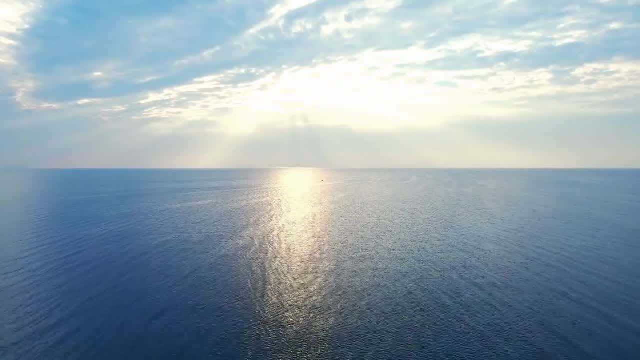 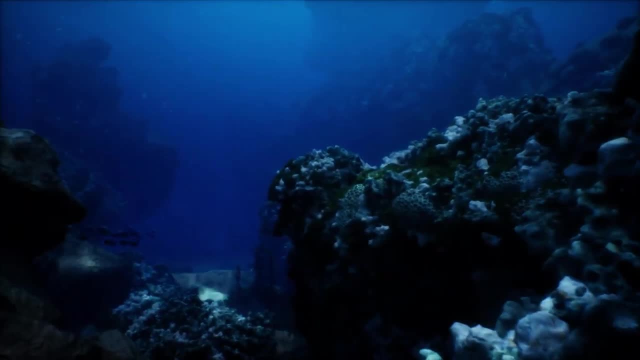 and lakes that we use and enjoy actually make up less than 0.01% of the total water on the planet. When it comes to the marine environment, these aquatic areas have high levels of dissolved salt and include the open ocean, deep sea, ocean and coastal marine ecosystems like coral reefs and. 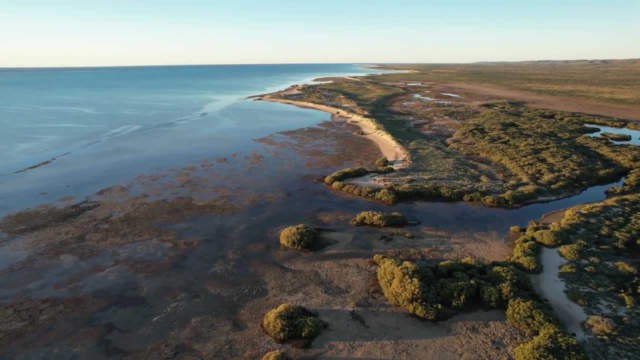 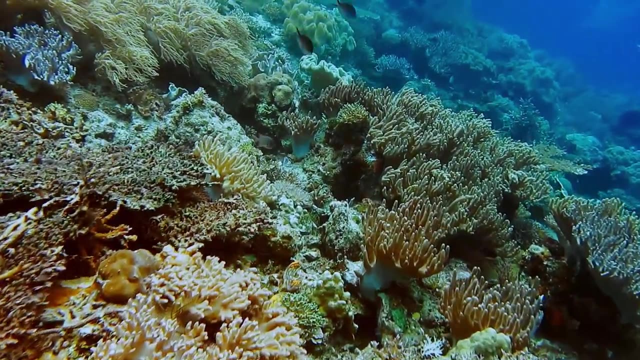 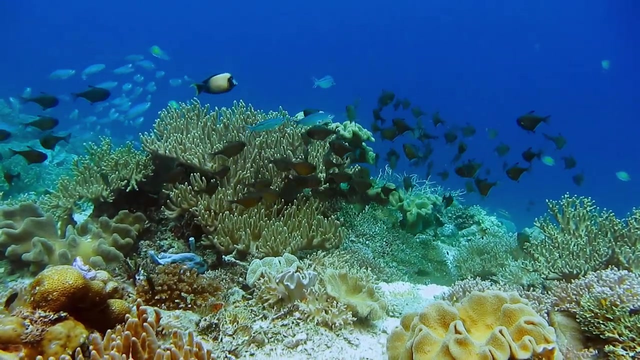 estuaries where tides meet streams, Each has different physical and biological characteristics. Coral reefs, for example, are incredibly diverse marine ecosystems, which in total, may account for a quarter of all ocean species alone. Corals are slow-growing, taking a long time to form. 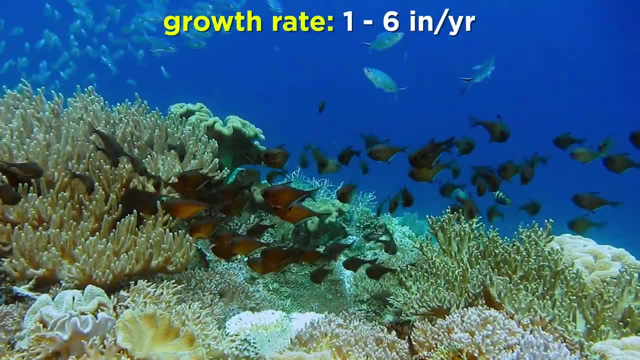 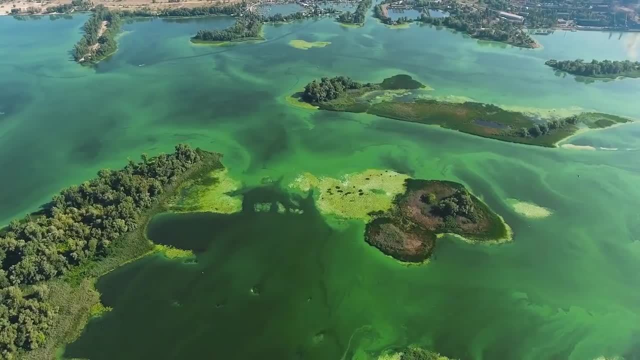 The fastest-growing coral grows 6 inches per year, but most grow less than an inch per year. Marine algae supply much of the world's oxygen- Think of it as the rainforest of the sea- And it absorbs a large amount of atmospheric carbon. 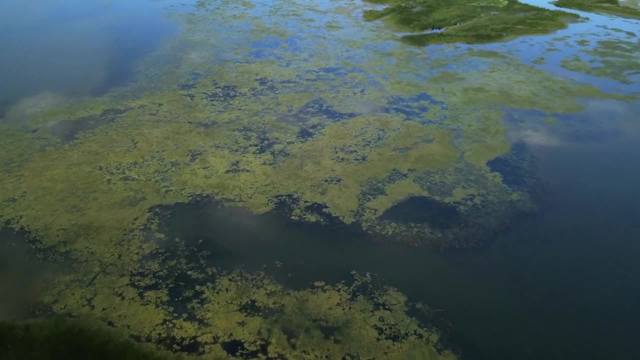 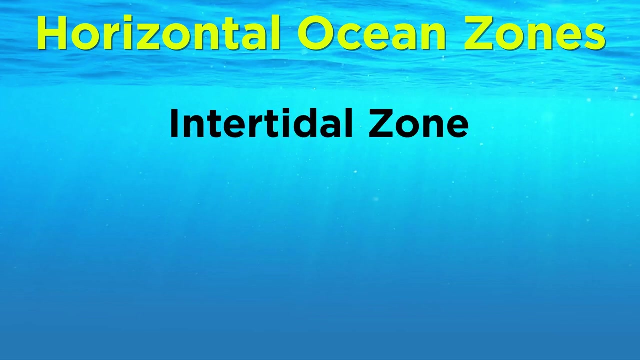 dioxide, which is increasing in amount year by year due to human-caused climate change. Within the ocean, we have four horizontal zones: the intertidal, pelagic, benthic and abyssal. We discussed these in the geology series, so let's just briefly review. 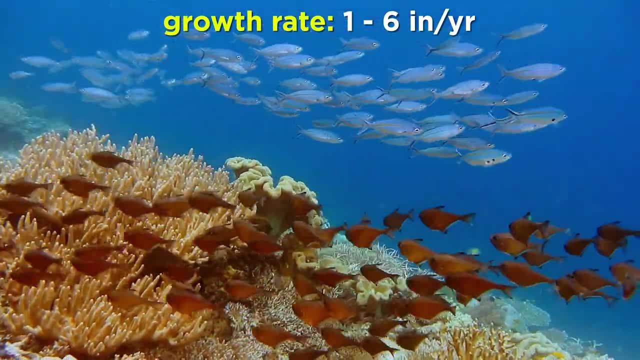 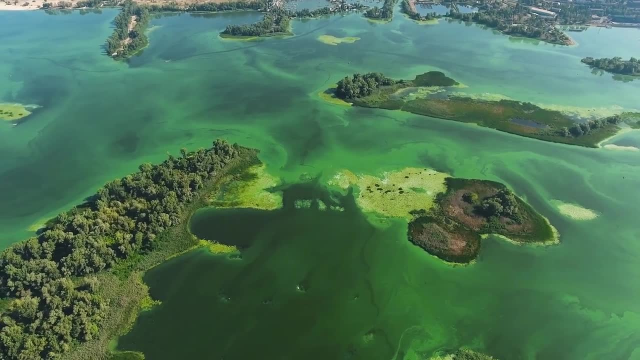 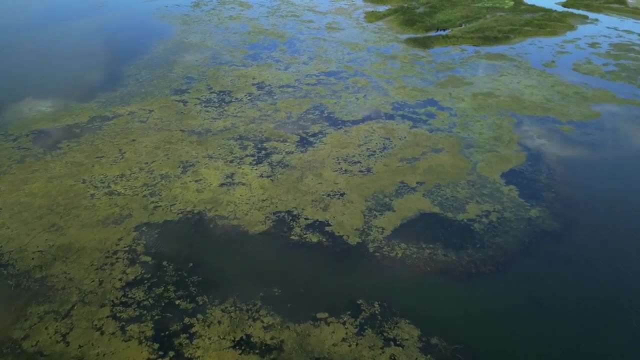 per year, but most grow less than an inch per year. Marine algae supply much of the world's oxygen- think of it as the rainforest of the sea- and it absorbs a large amount of atmosphere- carbon dioxide- which is increasing in amount year by year due to human-caused climate change. 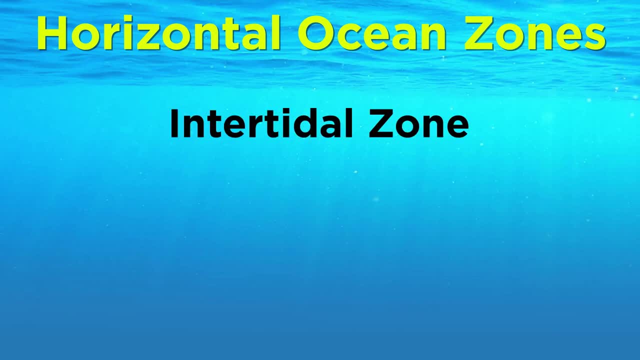 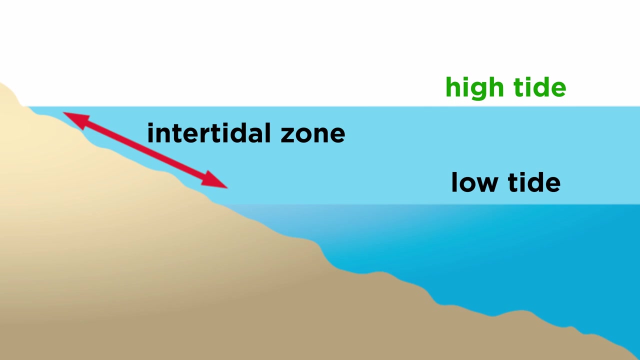 Within the ocean we have four horizontal zones: the intertidal, pelagic, benthic and abyssal. We discussed these in the geology series, so let's just briefly review. The intertidal zone is where the ocean meets the land. It is sometimes submerged and sometimes 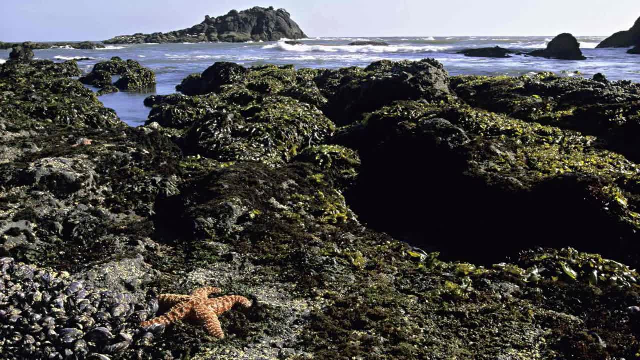 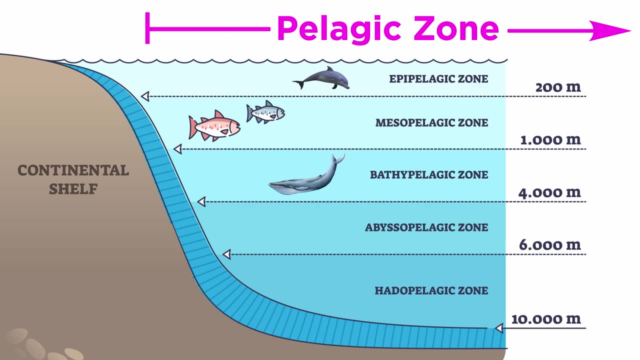 exposed as waves and tides come in and out. This zone can be rocky and act as home to algae, mollusks, snails, crabs, starfish and small fish. The pelagic zone is further from land and home to many more species of fish, as well as mammals like whales. 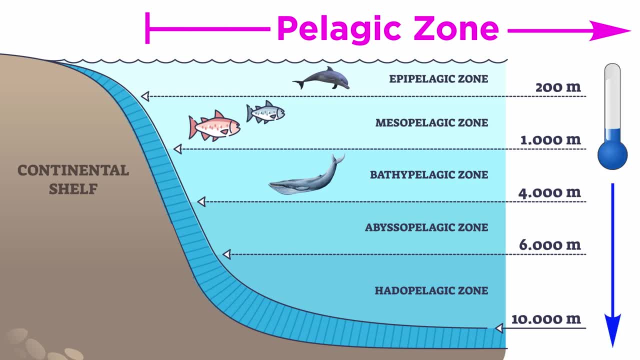 and dolphins. This region is colder and temperature varies at different depths due to thermal stratification or a separation of waters, due to varying temperatures and densities and the mixing of warm and cold currents. Next is the benthic zone, which includes the seafloor consisting of sand, silt and dead. 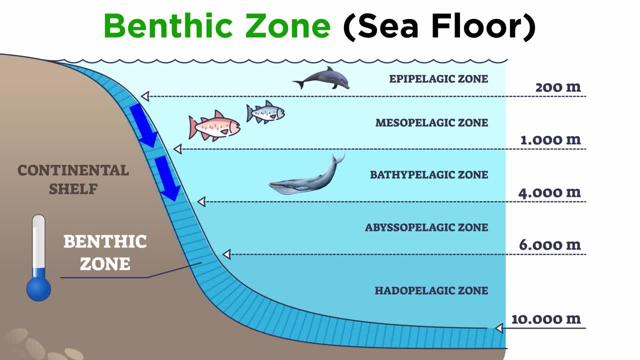 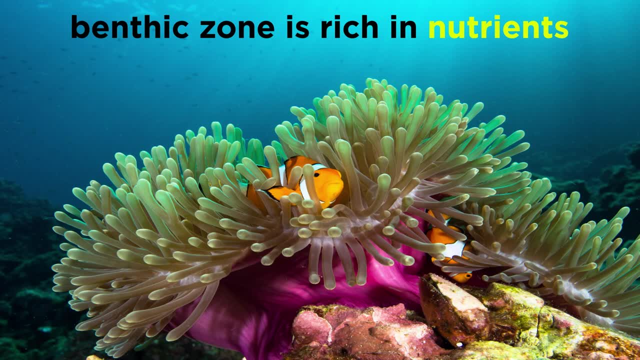 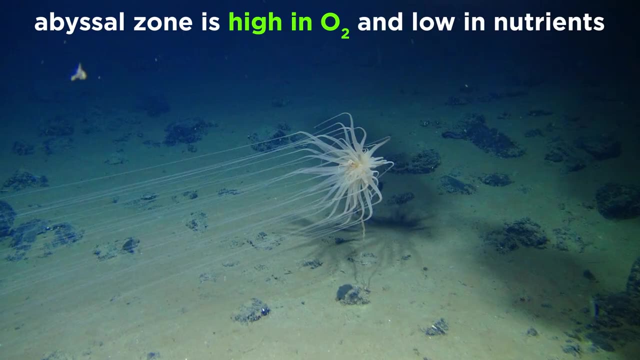 organisms. The temperature here is quite cold and decreases with depth while approaching the abyssal zone, the deepest part of the ocean. While the benthic zone is rich in nutrients supporting bacteria, fungi, sea anemones, marine worms and more, the abyssal zone, 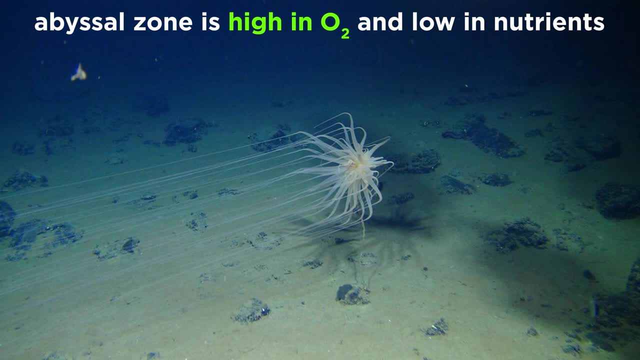 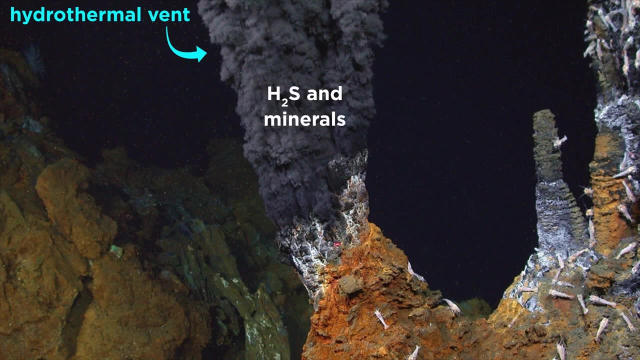 while high in oxygen, is low in nutrients. However, it's home to a unique ecosystem. Openings in the seafloor called hydrothermal vents emit large amounts of hydrogen sulfide and other minerals that support several types of chemosynthetic bacteria. These bacteria do not use sunlight for food, but rather derive their energy from. 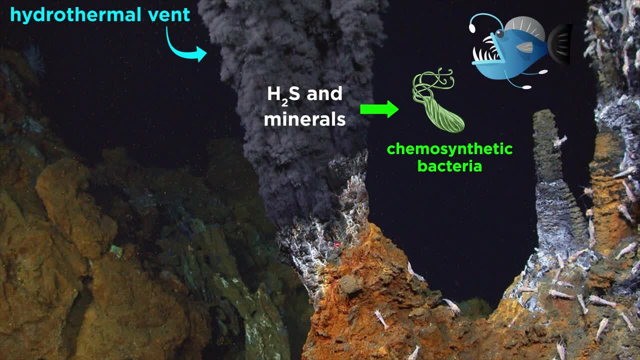 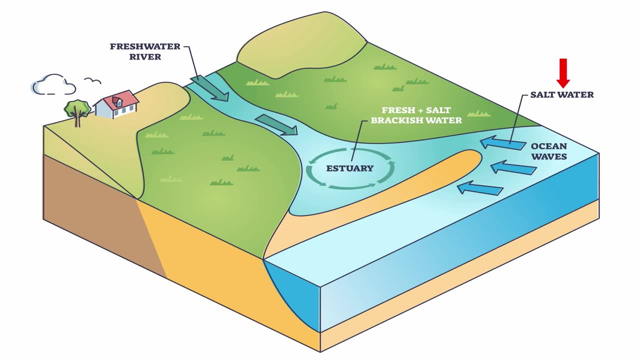 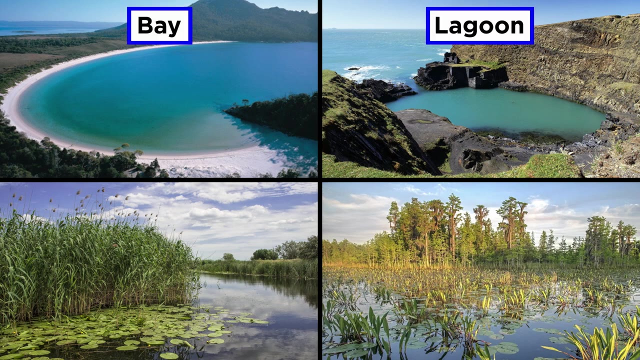 reactions involving inorganic chemicals. This, in turn, provides food for invertebrates and fish at these depths. Then there are estuaries, where saltwater from the ocean mixes with freshwater from the land. You may also know estuaries as bays, lagoons, wetlands and swamps. 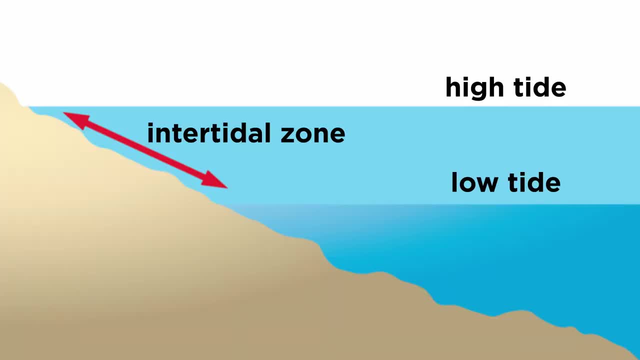 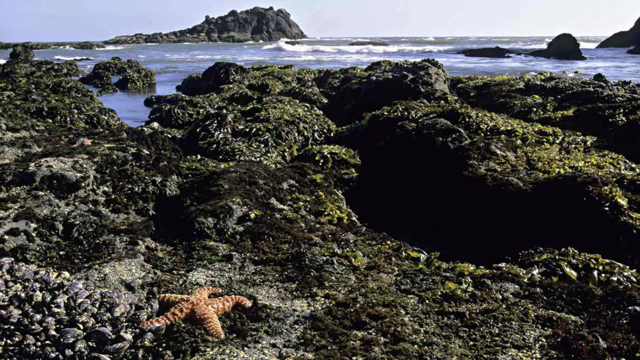 The intertidal zone is where the ocean meets the land. It is sometimes submerged and sometimes exposed as waves and tides come in and out. This zone can be rocky and act as home to algae, mollusks, snails, crabs, starfish and small fish. The pelagic zone is further from land and 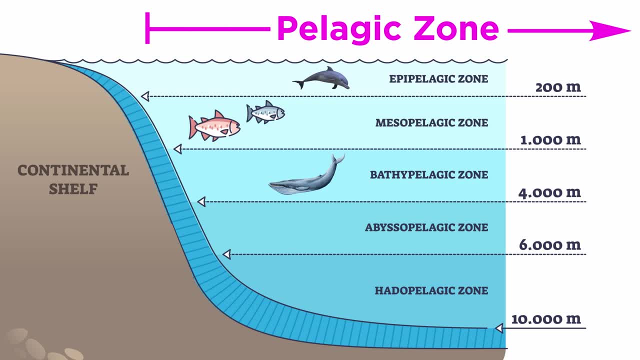 home to many more species of fish, as well as mammals like whales and dolphins. This region is colder and temperature varies at different depths due to thermal stratification or a separation of waters due to varying temperatures. The intertidal zone is where the ocean meets the 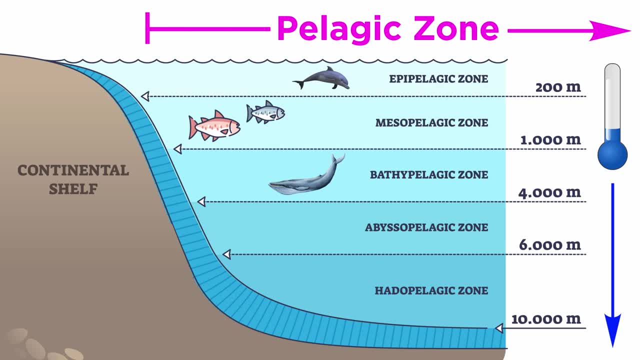 sea, and the sea is rich in nutrients and temperature and densities and the mixing of warm and cold currents. You can find a lot of seaweed here. Next is the benthic zone, which includes the seafloor consisting of sand, silt and dead organisms. The temperature here is quite cold and decreases. 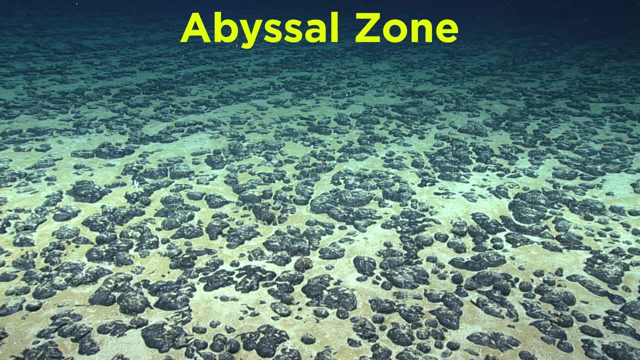 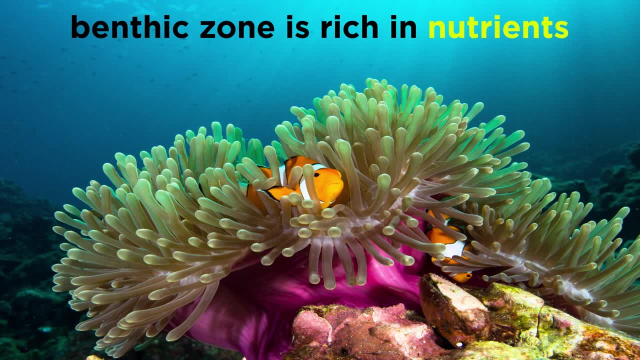 with depth while approaching the abyssal zone, the deepest part of the ocean. While the benthic zone is rich in nutrients supporting bacteria, fungi, sea anemones, marine worms and more, it is also rich in minerals, and it is also rich in minerals, and it is also rich in minerals. and. 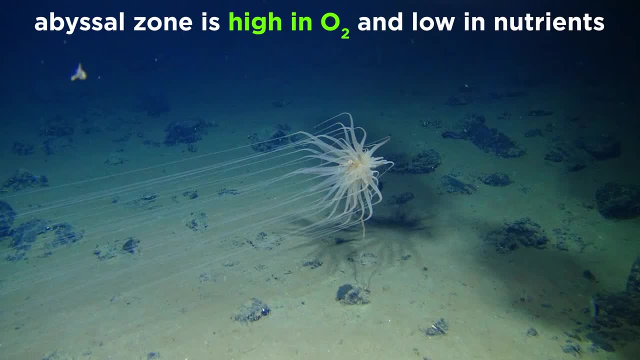 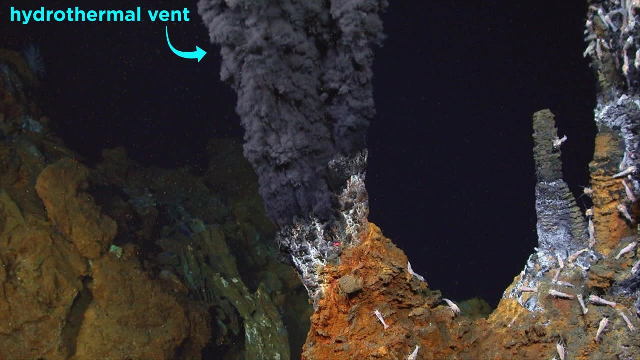 the abyssal zone. while high in oxygen is low in nutrients. However, it is home to a unique ecosystem. Openings in the seafloor called hydrothermal vents emit large amounts of hydrogen sulfide and other minerals that support several types of chemosynthetic bacteria. 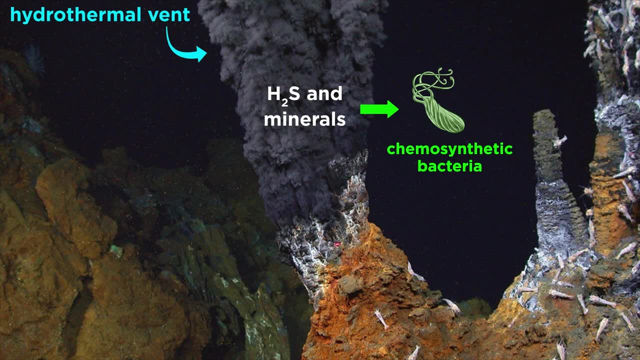 These bacteria do not use sunlight for food, but rather derive their energy from reactions involving inorganic chemicals. This, in turn, provides food for invertebrates and fish at these depths. Then there are estuaries where saltwater from the ocean mixes with 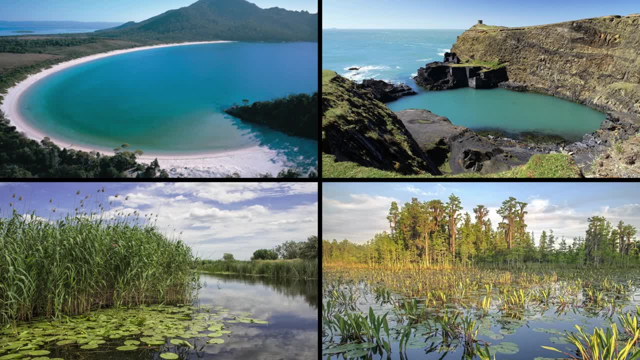 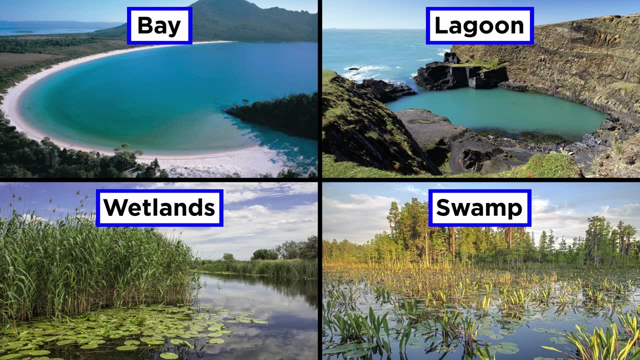 freshwater from the land. You may also know estuaries as bays, lagoons, wetlands and swamps. These ecosystems are adapted to cope with the challenge of the rise and fall of tides, as well as variations in water chemistry, primarily salinity. 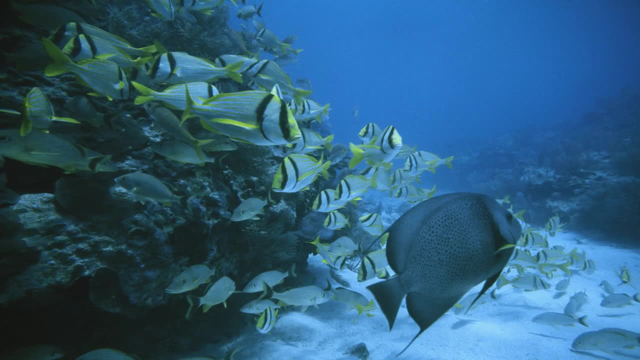 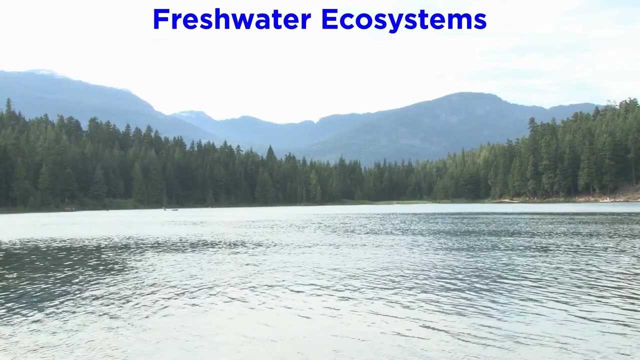 Despite this, estuaries are one of the most productive ecosystems on Earth, home to fish, shellfish, crustaceans, algae, plankton and mangrove trees. Numerous animals rely on estuaries for nesting and breeding grounds. Freshwater ecosystems include surface features. 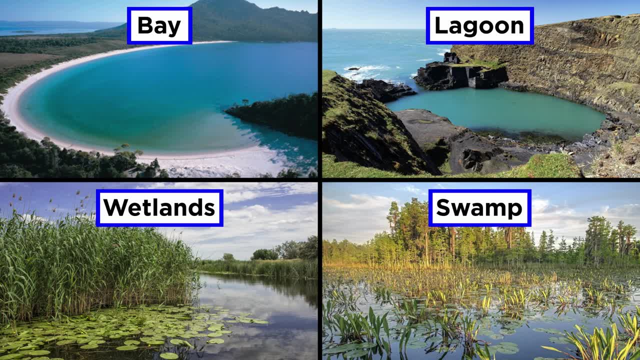 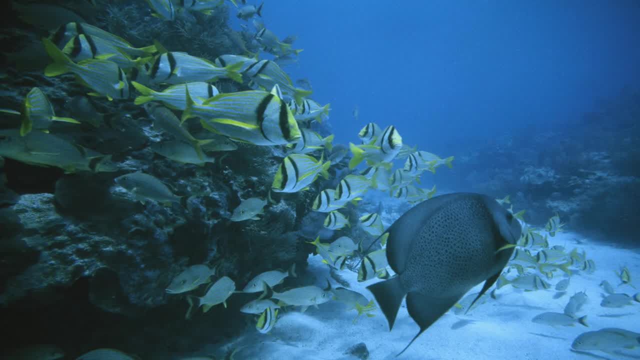 These ecosystems are adapted to cope with the challenge of the rise and fall of tides, as well as variations in water chemistry, primarily salinity. Despite this, estuaries are one of the most productive ecosystems on Earth, home to fish, shellfish, crustaceans, algae, plankton and mangrove trees. 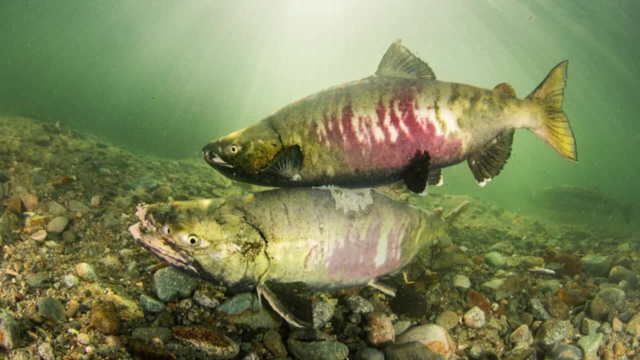 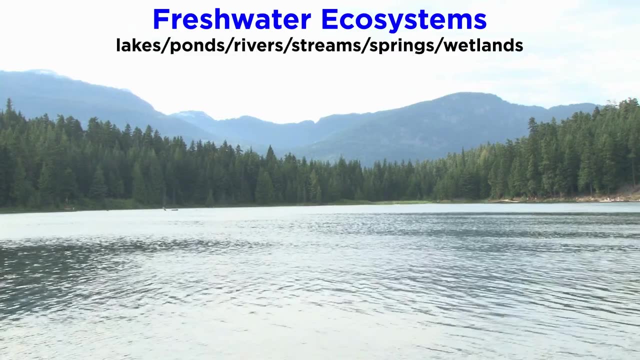 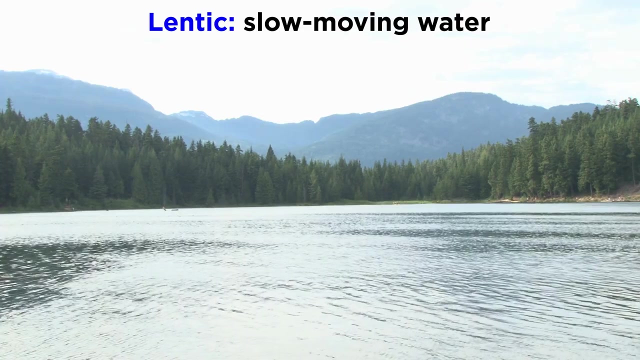 Numerous animals rely on estuaries for nesting and breeding grounds. Freshwater ecosystems include surface features like lakes, ponds, rivers, streams, springs and wetlands. They are either lentic, meaning slow-moving water like that found in lakes. 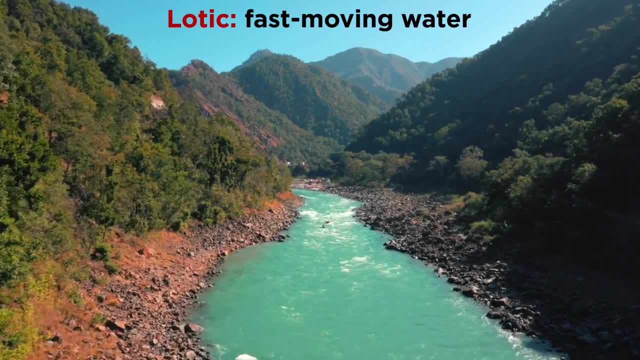 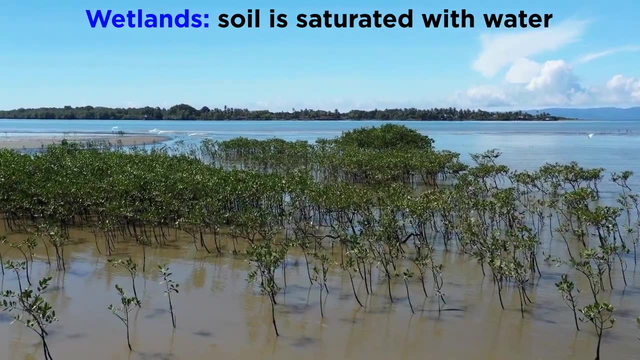 or lotic consisting of fast-moving water. like with rivers, Wetlands occur where soil is saturated or inundated with water for at least part of the time. They do not contain the same dissolved substances in the water as marine ecosystems, so the animals 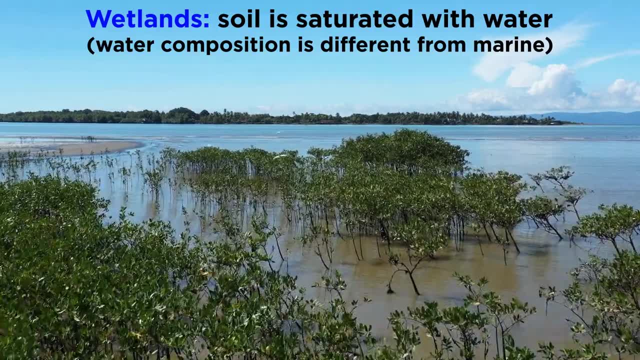 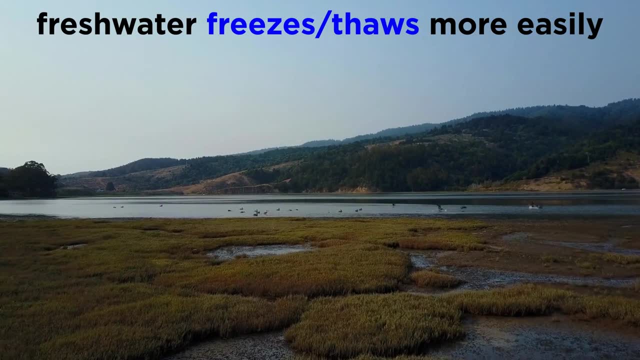 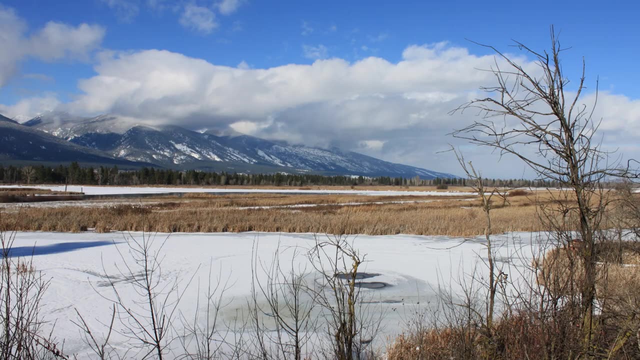 and plants living there would not survive in marine ecosystems without some serious and rapid adaptations. Because freshwater does not contain salt, it's more susceptible to freezing and thawing. Thus, freshwater plants and animals have adapted to survive this process. They have respiratory structures adapted specifically for freshwater and have evolved. reproductive and feeding behaviors for the rest of life. This is the end of the first part of the world, but at this point I mean the rest of the world. The rest of the world is not yet out of the question. What is real? What is real? That is what we know. The real question is: what is real, What is not real, What? 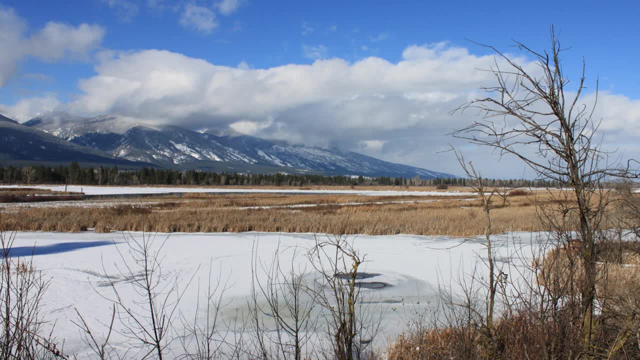 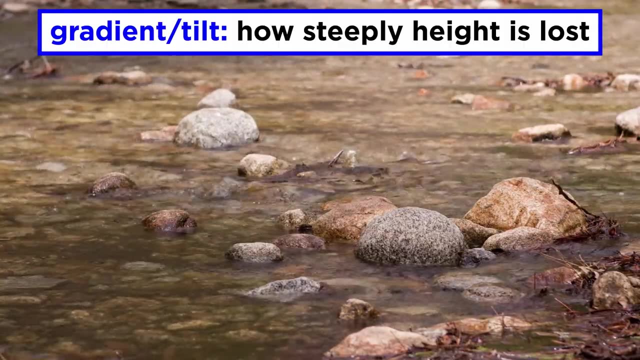 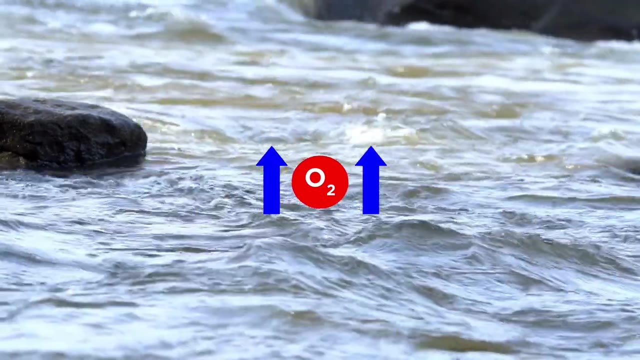 feeding behaviors that enable them to survive these temperature changes. The major zones in river ecosystems are determined by the riverbed's gradient or tilt, or by the velocity of the current. Faster moving turbulent water typically contains greater concentrations of dissolved oxygen, which supports greater biodiversity than slow moving water. 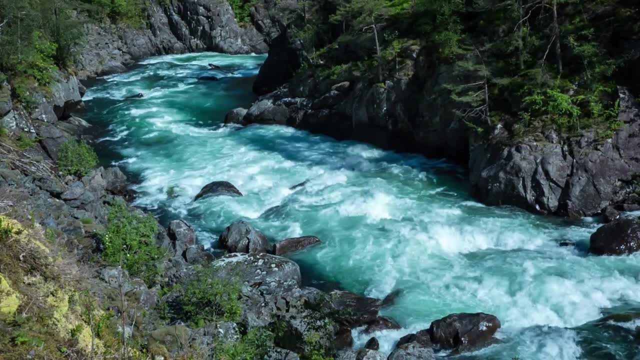 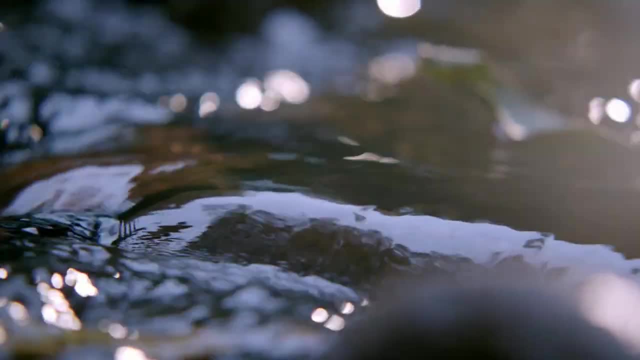 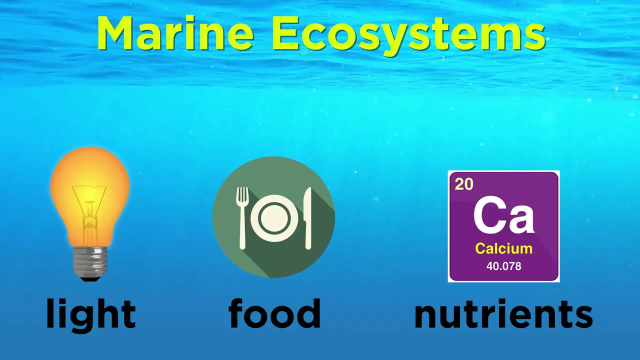 The ecology of running water thus is unique among aquatic habitats. due to unidirectional flow, a state of continuous physical change and a high degree of spatial and temporal micro-habitats at all scales, Marine ecosystems are characterized by factors such as availability of light, food and nutrients. 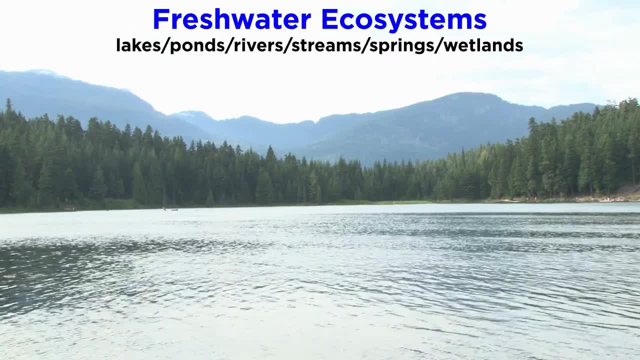 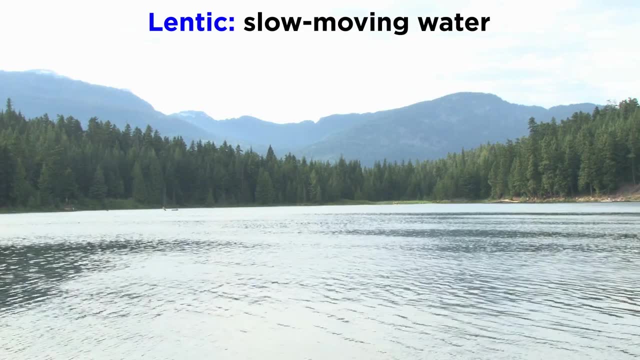 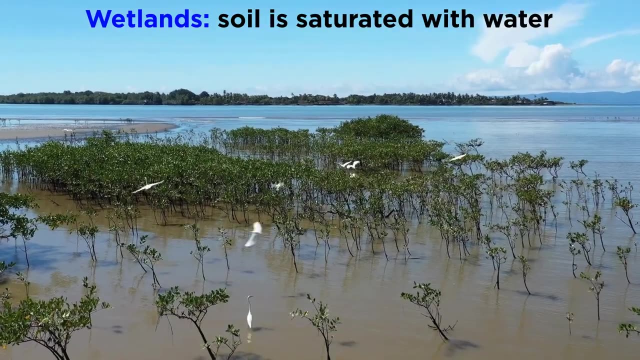 like lakes, ponds, rivers, streams, springs and wetlands. They are either lentic, meaning slow-moving water, like that found in lakes, or lotic, consisting of fast-moving water, like with saltwater. Wetlands occur where soil is saturated or inundated with water for at least part of the 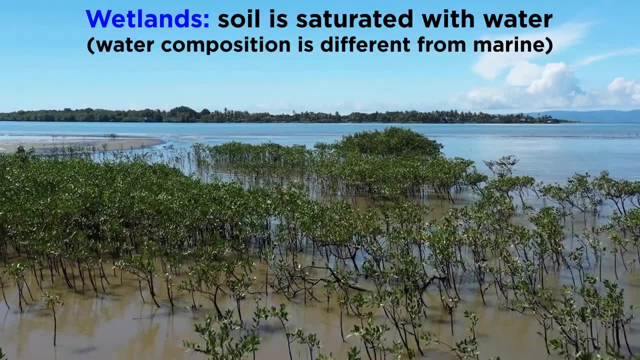 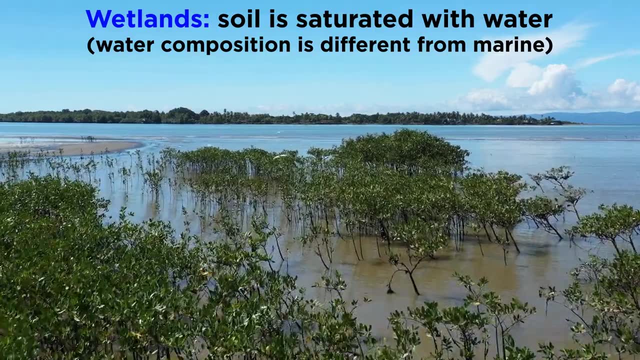 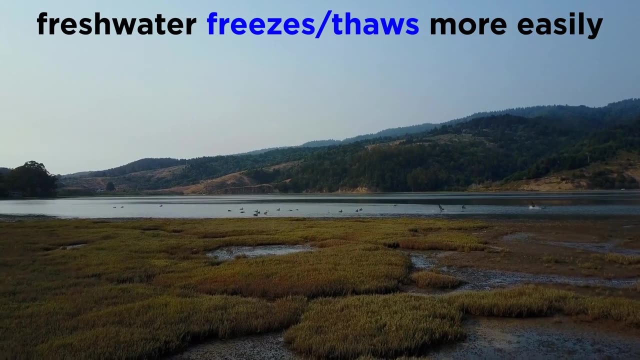 time. They do not contain the same dissolved substances in the water as marine ecosystems, so the animals and plants living there would not survive in marine ecosystems without some serious and rapid adaptations. Because freshwater does not contain salt, it's more susceptible to freezing and thawing. Thus, freshwater plants and animals have adapted to survive this process. 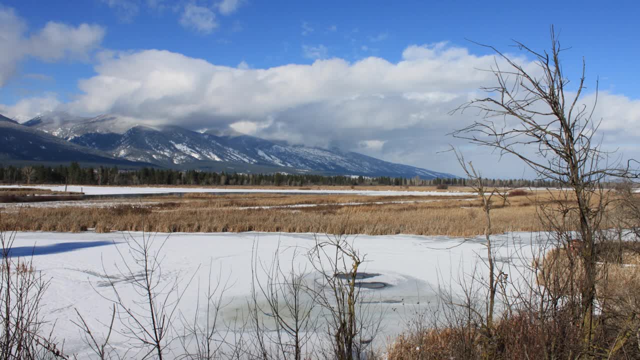 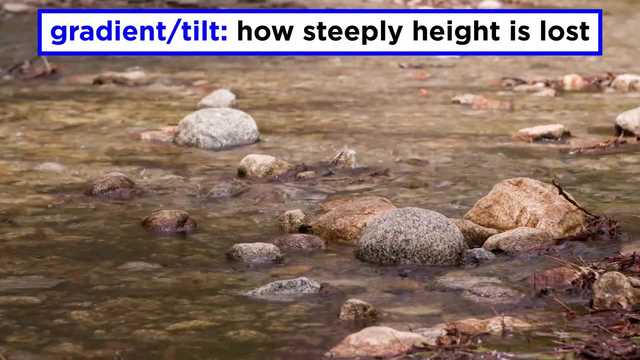 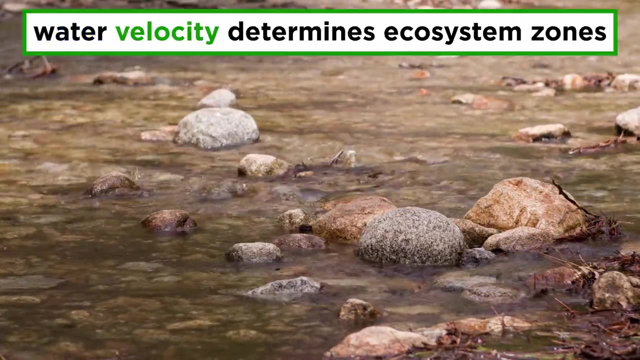 They have respiratory structures adapted specifically for freshwater and have evolved reproductive and feeding behaviors that enable them to survive these temperature changes. The major zones in river ecosystems are determined by the riverbed's gradient or tilt, or by the velocity of the current. Faster-moving, turbulent water typically contains greater 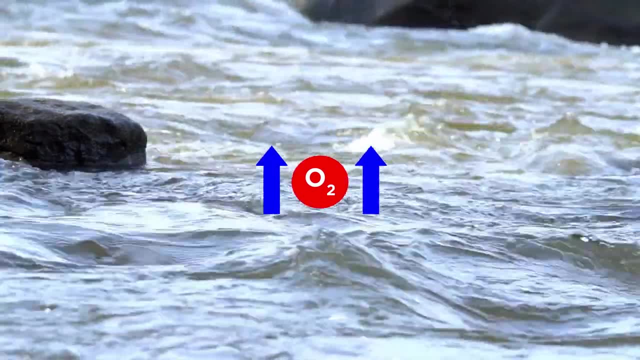 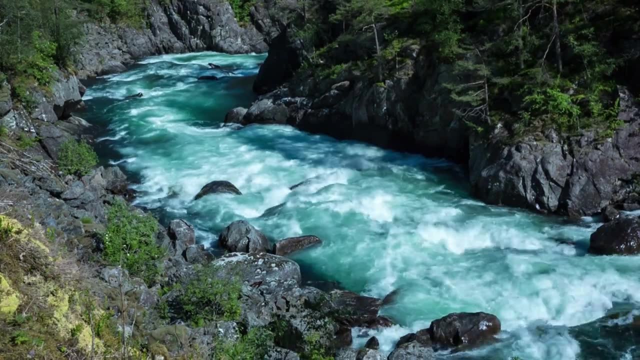 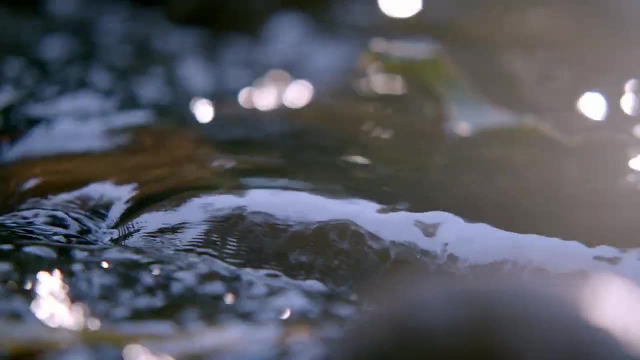 concentrations of dissolved oxygen, which supports greater biodiversity than slow-moving water. The velocity of running water thus is unique among aquatic habitats, due to unidirectional flow, a state of continuous physical change and a high degree of spatial and temporal microhabitats at all. 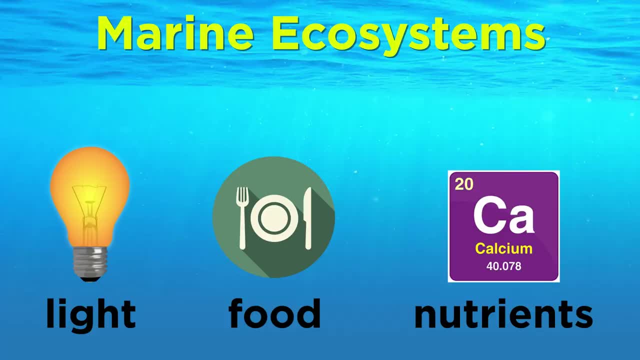 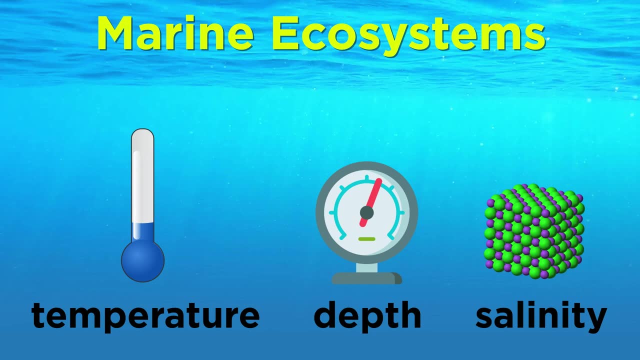 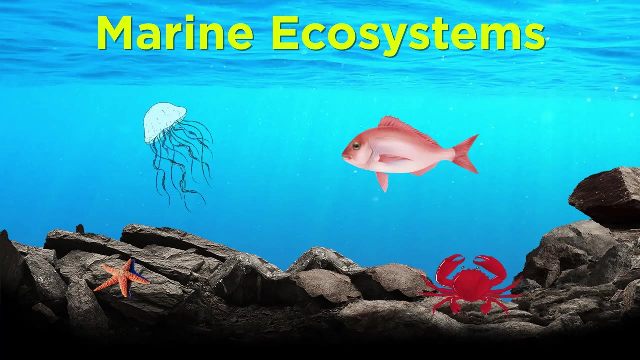 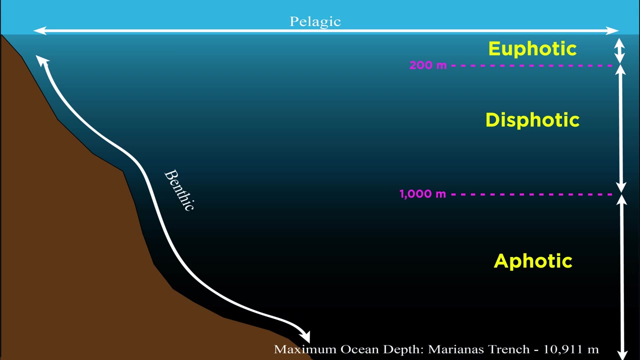 scales. Marine ecosystems are characterized by factors such as availability of light, food and nutrients. Other factors include water temperature, depth and salinity, as well as local conditions, can change the composition of species that make up the marine community In the ocean. the three vertical zones based on depth are the euphotic, dysphotic and aphotic zones. 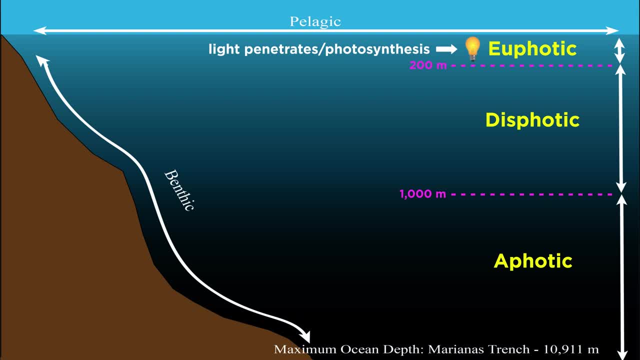 The euphotic zone is the area where light can penetrate and where the vast majority of photosynthesis takes place. It goes down about 200 meters. The middle layer is the dysphotic or twilight zone, where less light reaches. The third and deepest layer is the aphotic zone, and this layer is completely dark.